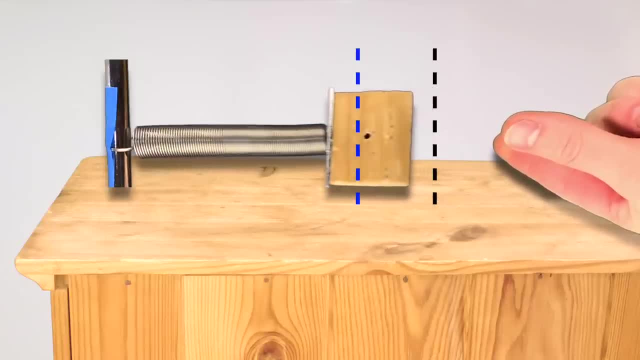 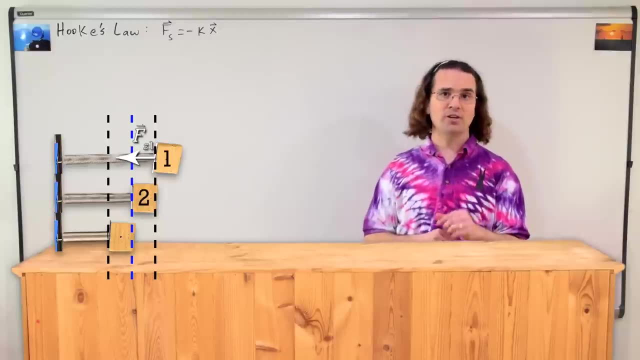 by the force of the spring. Notice, the mass passes through rest position and will go all the way over to the left. And let's pause it there for a moment. Let's call position 2, the location of the mass when it is at equilibrium position, and position 3,. 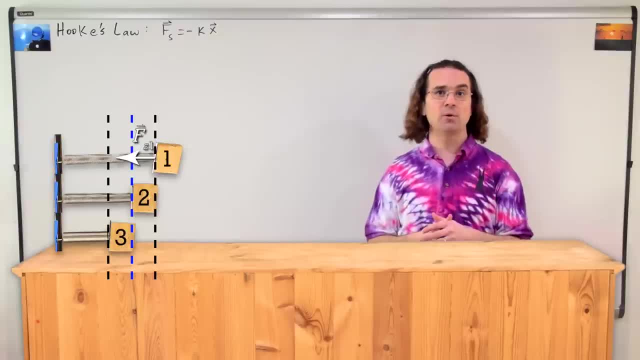 the location of the mass when it is at its maximum displacement from equilibrium position to the left? Olivia, what is the direction of the spring force on the mass when the mass is at position 2?? That question does not make any sense because the displacement from equilibrium position at 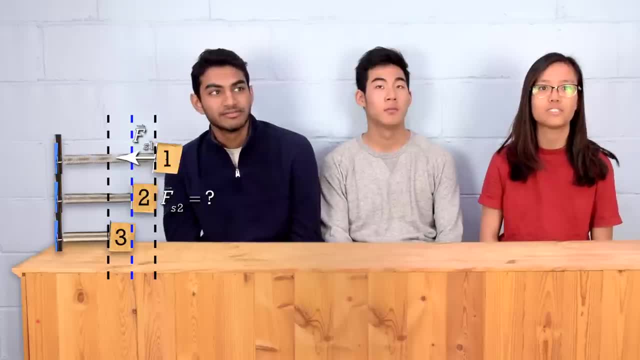 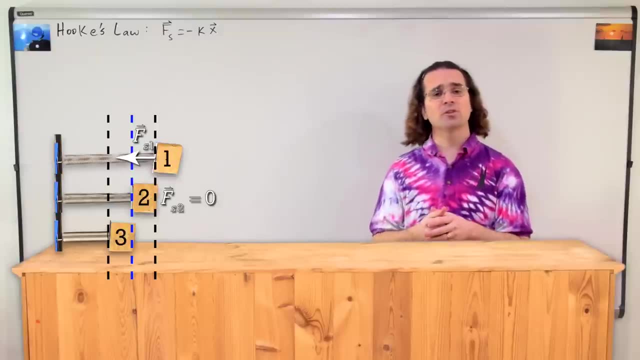 number 2 is 0. Therefore, according to Hooke's law, the force of the spring is also 0 and has no direction. That is correct, Olivia. Thank you, Kevin. what about the direction of the force of the spring? 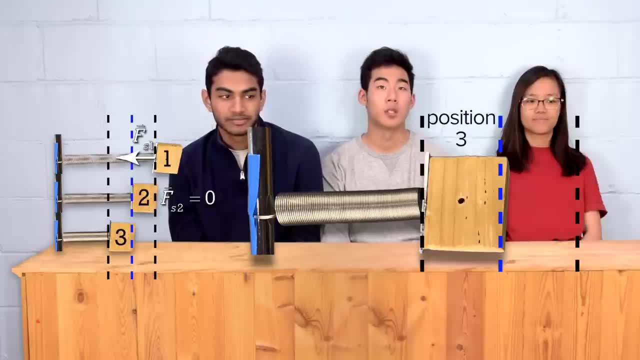 when it is at position 3?? At position number 3, the displacement of the mass from the rest position is to the left. Therefore, the force of the spring is to the right. That is also correct. Thank you, Kevin. Let's go back to the beginning of this demonstration for a moment and watch what happens. 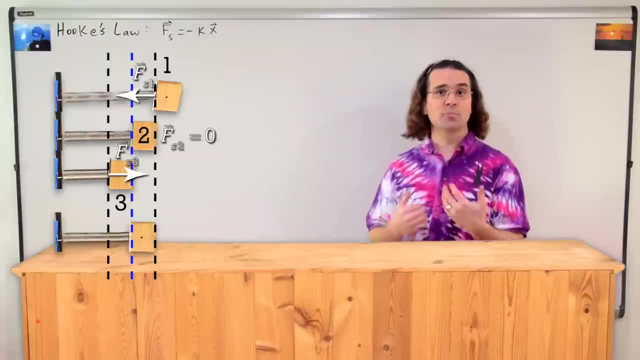 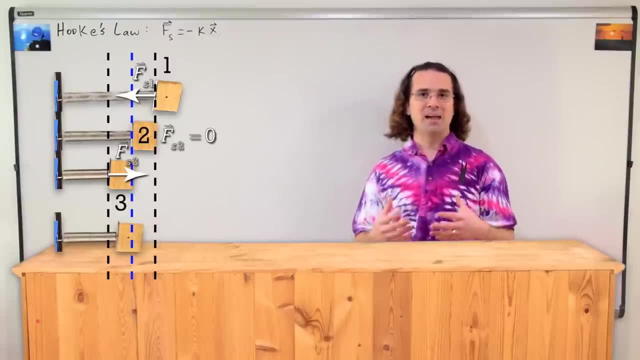 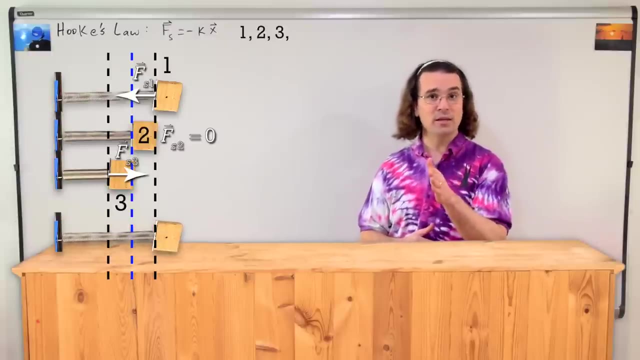 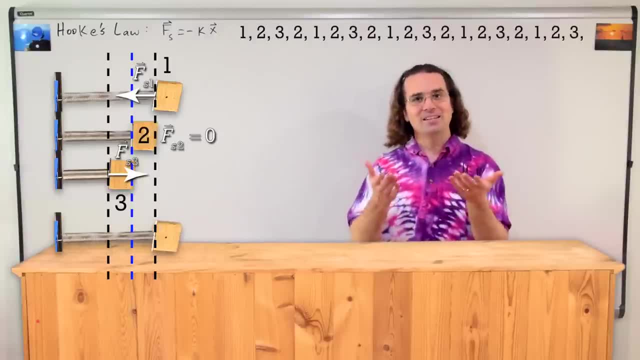 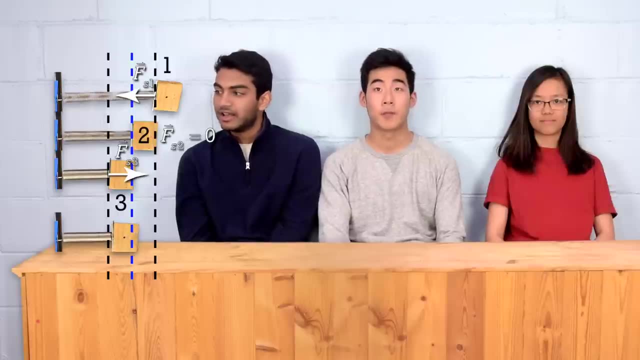 3, 2,, 1,, 2,, 3, and Kevin. in the absence of friction, when will the pattern of this mass spring system end? If there is no friction, it will never end. Correct? This is called simple harmonic motion. 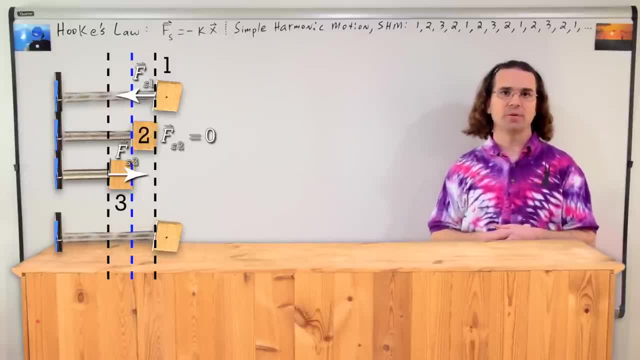 This mass spring system is in simple harmonic motion. It will continue to oscillate back and forth like this forever, in the absence of friction. There are two requirements for the force that cause simple harmonic motion. One is that this force causes the center of the 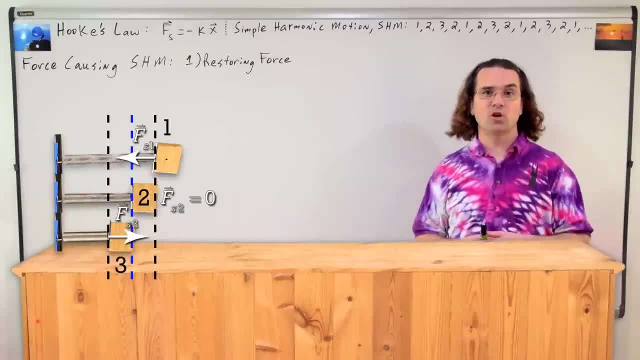 system to be directed towards the center of the system. The other is that this force causes the heart of the system to be directed toward the center of the system. So, in other words, the force of the motion First, the force causing simple, harmonic motion must be a restoring force.